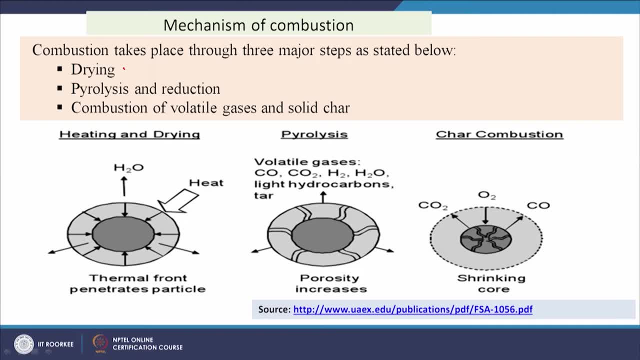 takes place through different steps: At first the drying, then pyrolysis and reduction and then combustion of volatile gases and solid char. So when we apply heat to the material in presence of oxygen, So at first the drying takes place, So at first the drying takes. 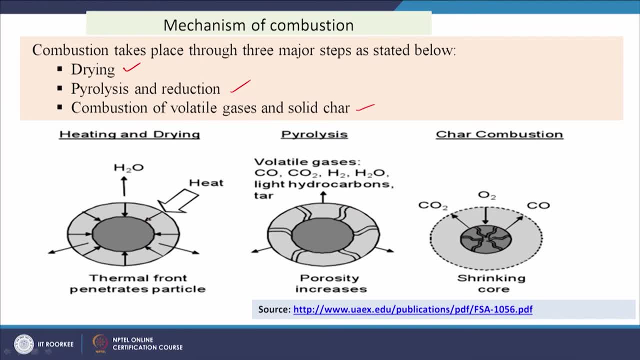 place. moisture goes off, Then the volatiles comes out from it, some of the solids and then the volatiles and the residual material. both are oxidized. So these are the different mechanism and with time the size of the particle- solid particle- reduces. So that is called. 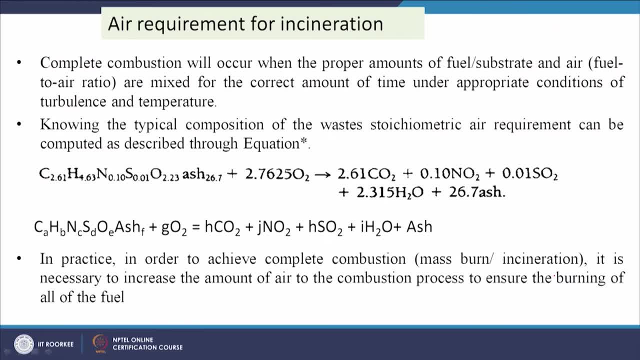 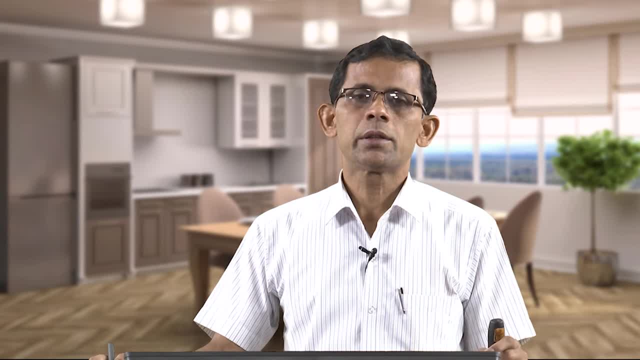 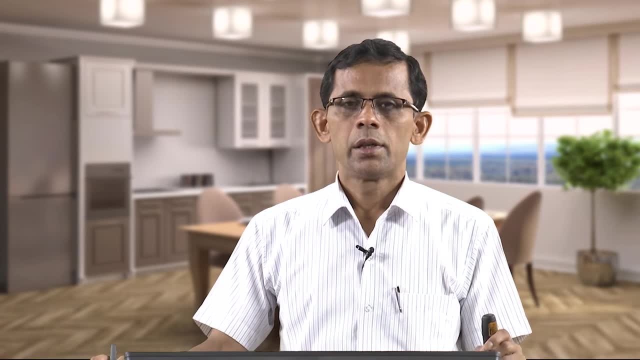 shrinking core model for the combustion. Now, what is the air requirement? How can you calculate? So you know the material will be having different components: carbon hydrogen, oxygen, nitrogen ash, etc. So its reaction and what are the different products will be produced. 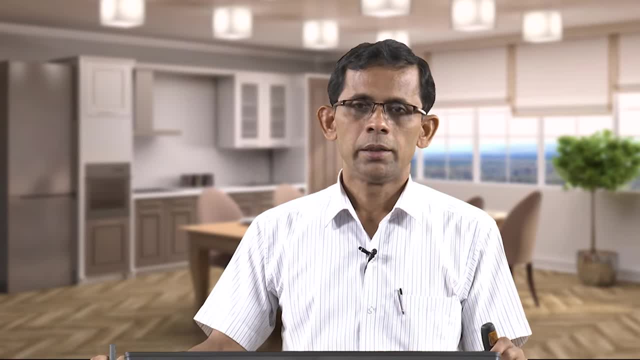 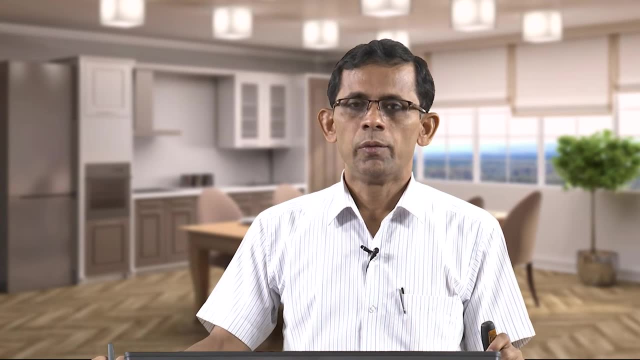 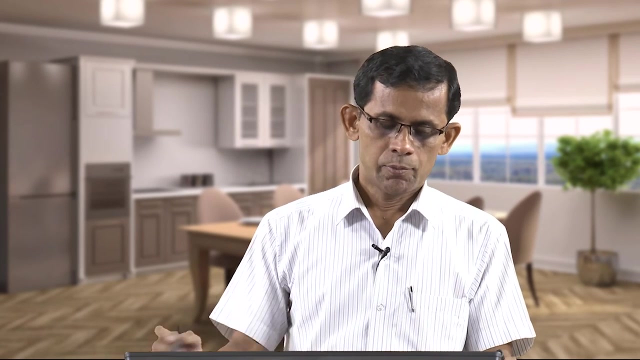 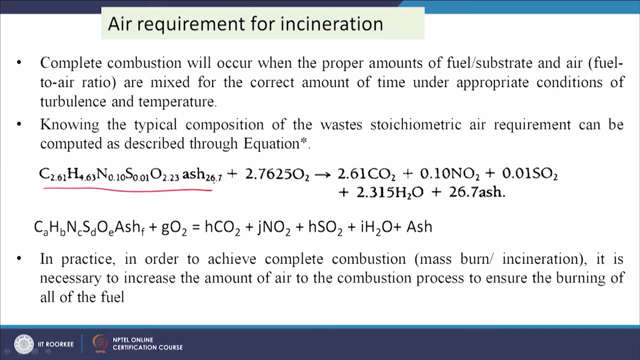 that is not so easy to predict. There is not a single component reaction, So heterogeneous material, so reactions will be difficult to predict. So we have to develop some empirical relationships like, say, if we have a waste materials, the molecular weight is known, that is, having carbon hydrogen, nitrogen, sulphur oxygen. 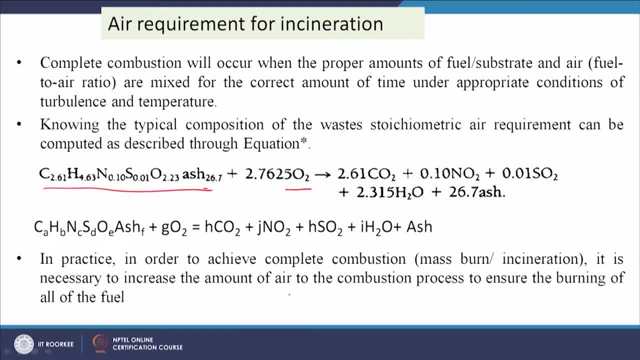 and ash, material that is reacting with some oxygen and then that will give us CO2, NO2, SO2, H2O and ash. So by regression, so doing set of experiments, by regression the people have developed this type of expression or we can generalize it like CA, HB, NC, SD, OE. 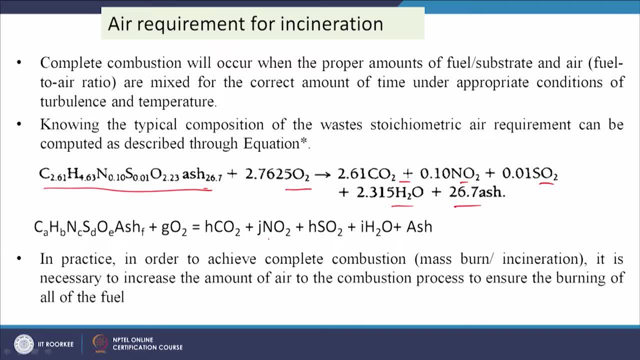 SF plus GO2 is giving us HCO2 plus JNO2 plus HSO2 plus IH2O plus ash and with the regression of the data, this A, B, C, D, E, F, G, H, J, H, I, J, I value can be Now, after the ultimate. 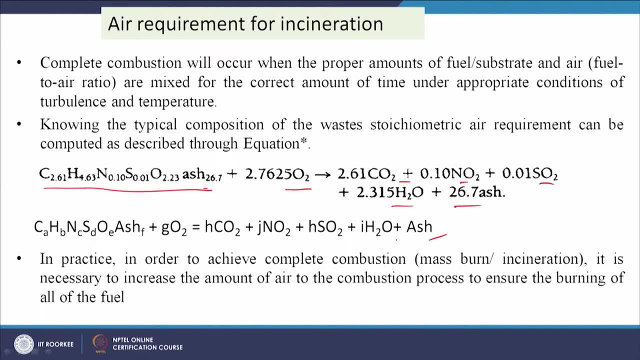 analysis of the feedstock or the waste material, the A, B, C, D, E, F, G, H, J, H, I, J, I value can be. We can say A, B, C, D, E and F also can be determining the ash content of it and its. 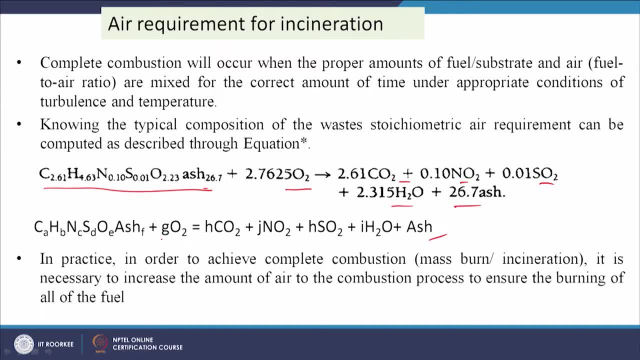 molecular mass and then considering these reactions and through mass balance, We can get the value of g, H, J, I, etcetera. We will be able to get the value of other coefficients We can get What is the value Next? 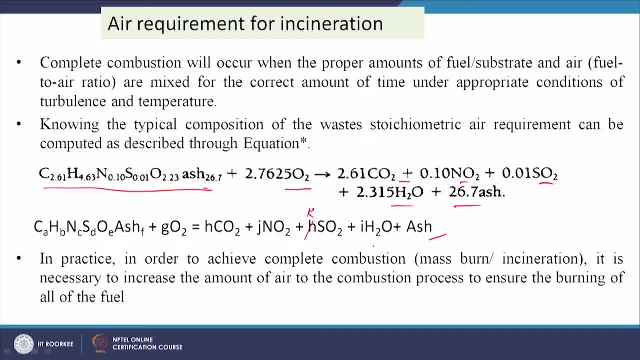 I etcetera the. in practice, in order to achieve complete combustion- that is called mass burn or incineration, it is necessary to increase the amount of air to the combustion process to ensure the burning of all the fuel. So these reactions stoichiometrically. some oxygen requirement is there, but if we provide 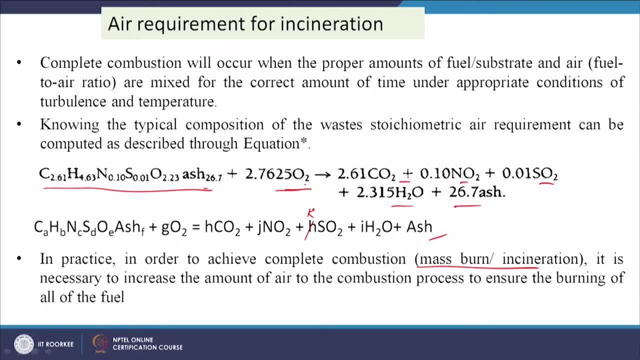 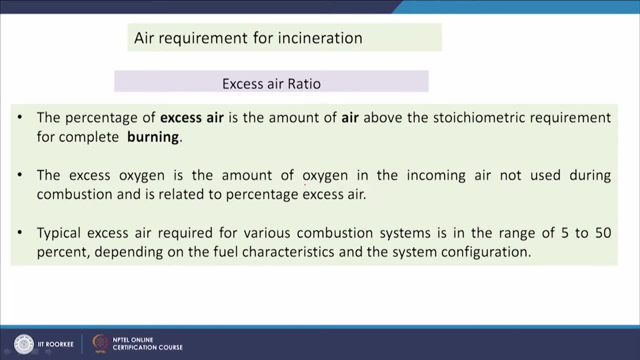 this oxygen. so complete combustion will not get. always some excess oxygen or air has to be provided And there is one excess air ratio: the air which will not be used, the oxygen which will not be used. with respect to the total air or oxygen supplied, that will be the excess. 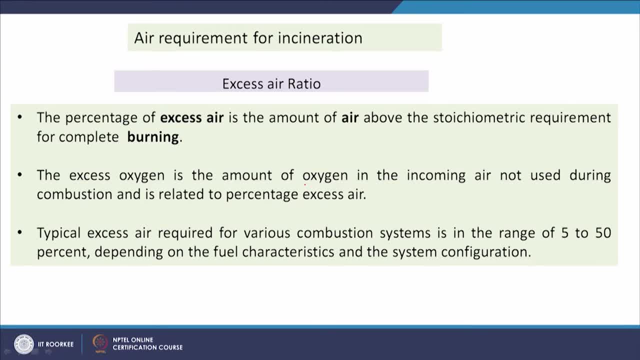 air ratio and it has been seen that the excess air requirement ratio requirement varies from 5 to 50. it has been found that typical excess air required for various combustion system is in the range of 5 to 50 percent, depending on the fuel characteristics and the system. 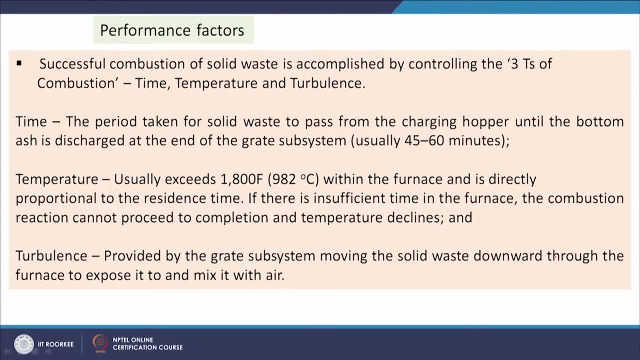 condition And the performance of the combustion reactions depends upon three T's, basically three T's, that is, time, temperature and turbulence. so when we are interested to heat it and combust it, we need to provide certain time so that complete conversion can take place within that time, as per the rate constant of the reactions or as per the rate of the reactions. 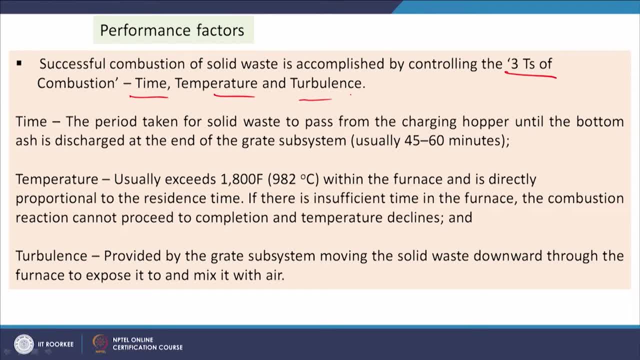 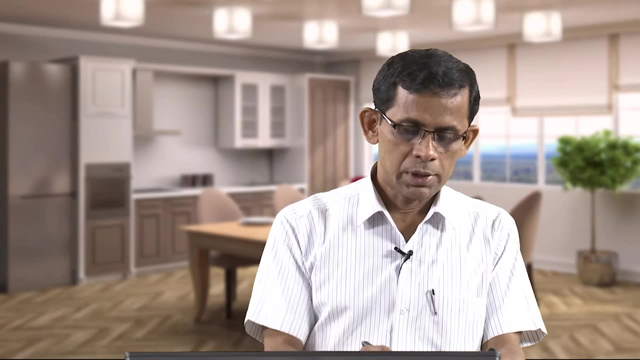 and then Temperature. certainly certain temperature is required for firing itself and to maintain the rate of reactions. and then turbulence is needed, because turbulence will give us more chance of the mixing of the air and the solid particles. So this time temperature and turbulence are most important parameters which influence 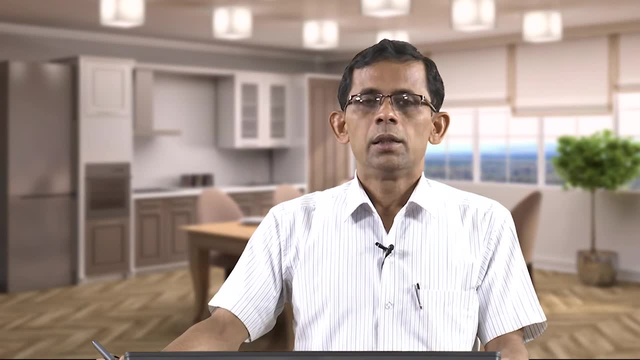 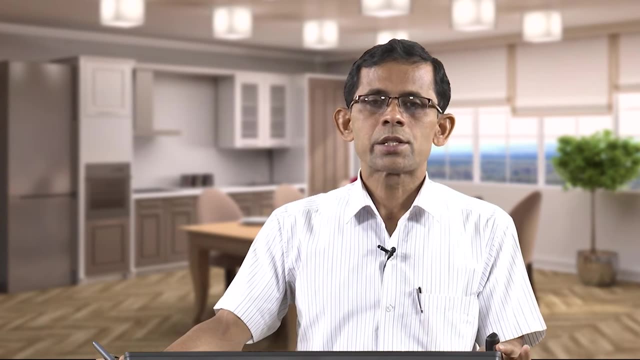 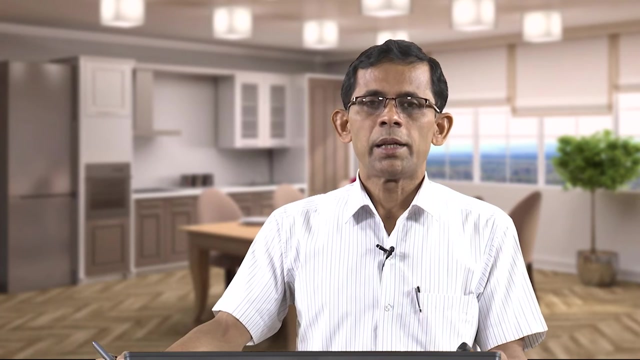 the performance, and that can be optimized also and to improve the performance of the combustion process. So here we are talking of structural type of combustion equipment. so here theどうの さつまいのありとして that the state and the buildings we want to have the 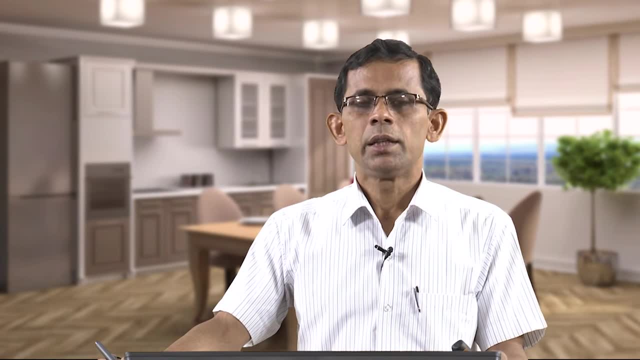 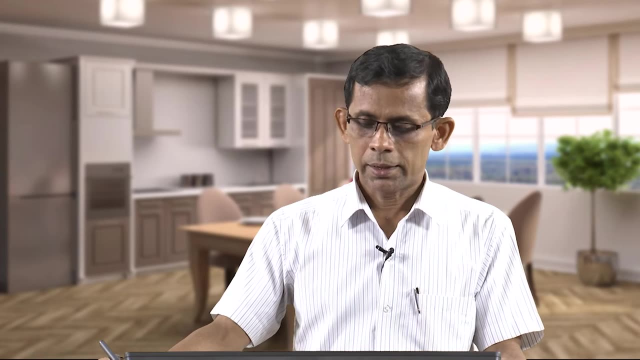 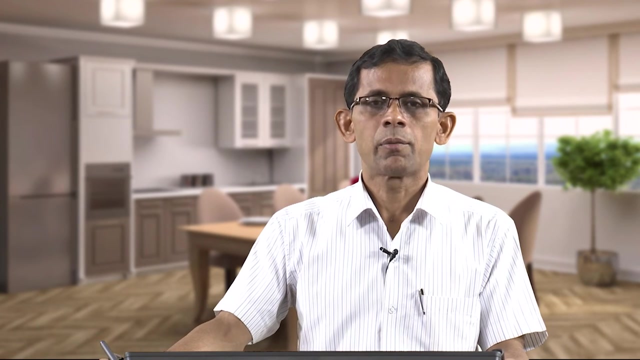 body of which are actually designed to be a temperature, in which the temperature at the moment will determine the body temperature. A, T, x is basically temperature we want to give to the engine which is in the atmosphere. it is probably seen in the the reference image of internal parts like these. 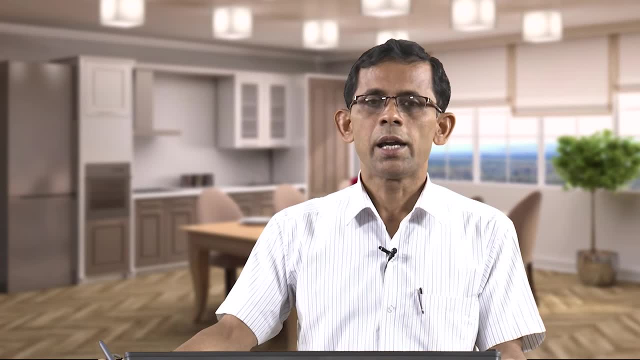 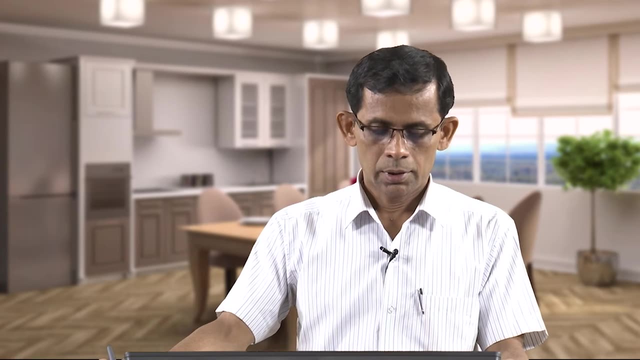 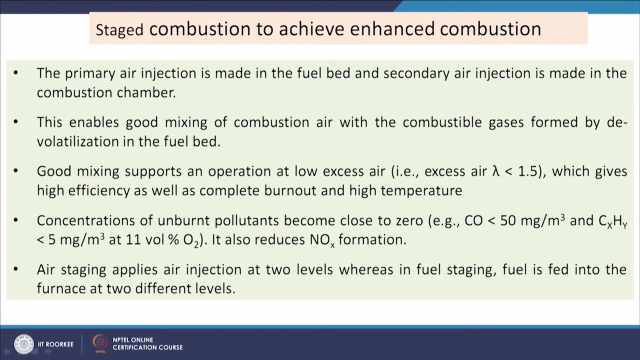 biomass. in that case we will be using initially high value of oxygen and then, in the subsequent step, lower value of the oxygen. the air ratio will be less And we see that air we are providing in the first step is the primary air and the second step, when we are providing it, is secondary air. So the primary air injection is made. 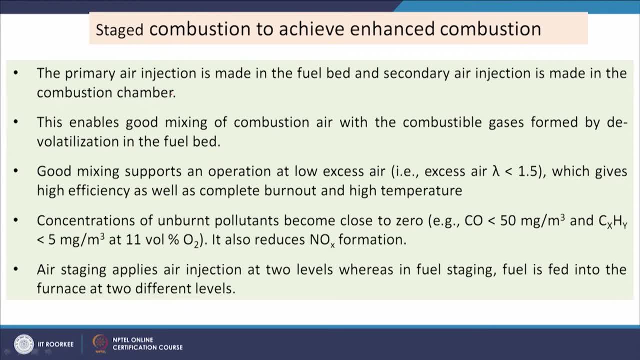 in the fuel bed and secondary air injection is made in the combustion chamber and this enables good mixing of combustion air with the combustible gases formed by the debolatilization in the fuel bed and good mixing supports and operation at low excess air that is lambda. 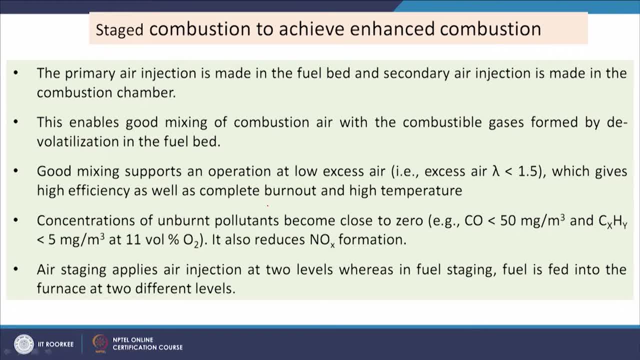 value less than 1.5, which gives high efficiency as well as complete burnt out and high temperature. Concentrations of unburnt pollutants become close to 0 in this case, and air staging applies air injection at two levels, whereas in fuel staging 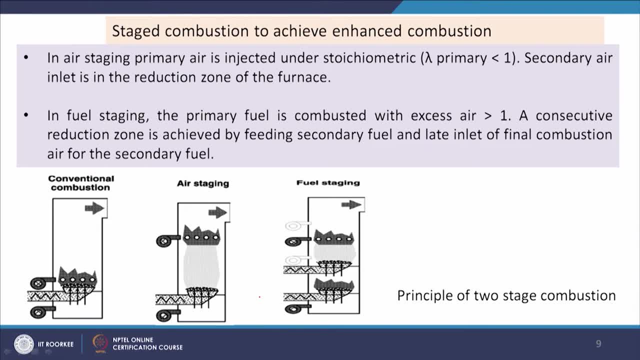 Fuel Fuel. Fuel Fuel is fed into the furnace at two different levels. So here we see that it is conventional combustion and here air staging. So air is provided here primary and this is secondary air and fuel staging. So here we are providing primary air and then secondary air, and again 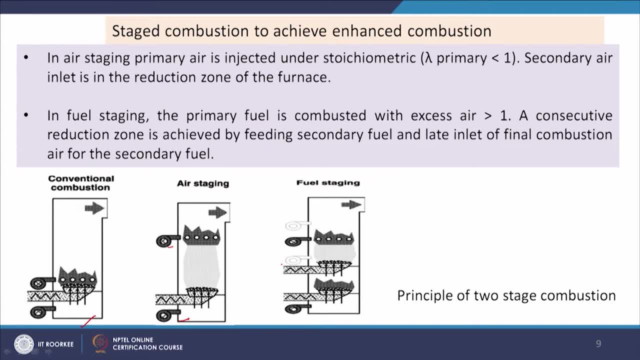 we are providing the feed also, So that way different steps or stages can be implemented for the combustion. Then air can be produced. So first stageення to primary catador. one reduction. 냄새gsma во asked eupof thee. лег enc. yhto conjecturebersaza wes hai the Alexis huvennis. In the same upgraded to the air used as the third phase in phase of the foundation. It is therefore the primary air injected is injected under stosometric ratio and secondary 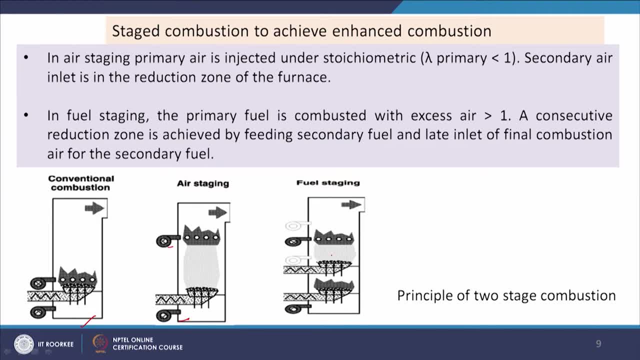 air inlet is in the reduction zone of the furnace and then fuel staging is completed with X s air greater than 1 lambda value, greater than 1a conseguarto be reduction zone is achieved, achieved by feeding secondary fuel here and later some final combustion air is provided. 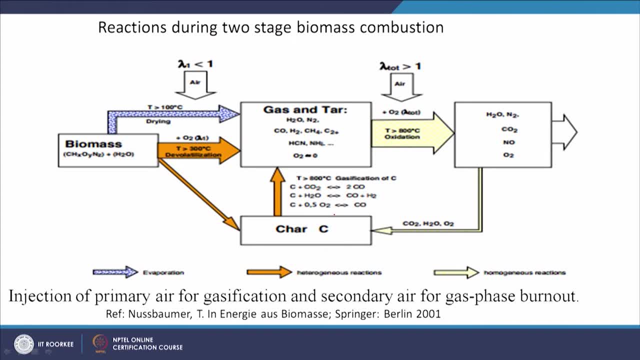 for the secondary fuel And these are the different reaction schemes. so waste and biomass is coming here, so that is first you. gas and tear is produced and the remaining is your char. so there will be some combustion. so oxygen provided, here lambda, 1 less than 1 less, and here secondary are more than this 1.. 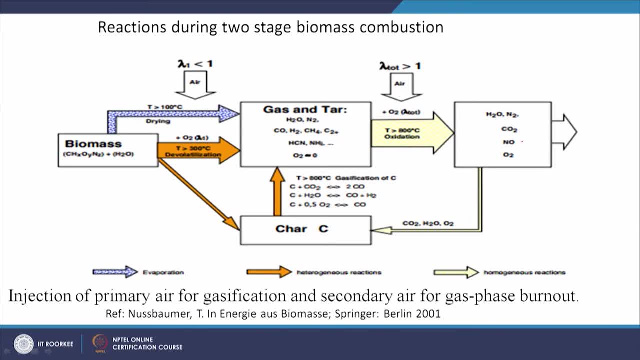 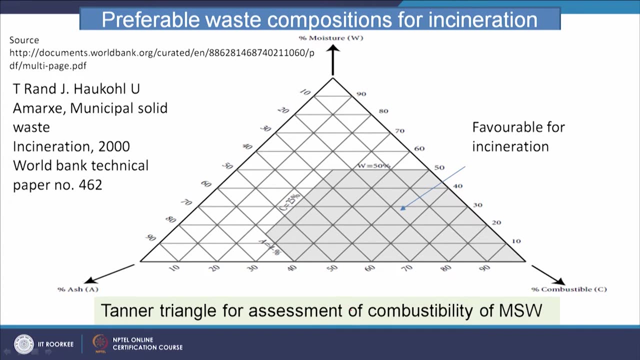 So here there will be reactions: NOx, CO2, O2 will be available in excess also, so that will be reacting with the char, and this type of reactions will go on. So a number of reactions will take place simultaneously in the combustion chamber and this slide shows us the selection. 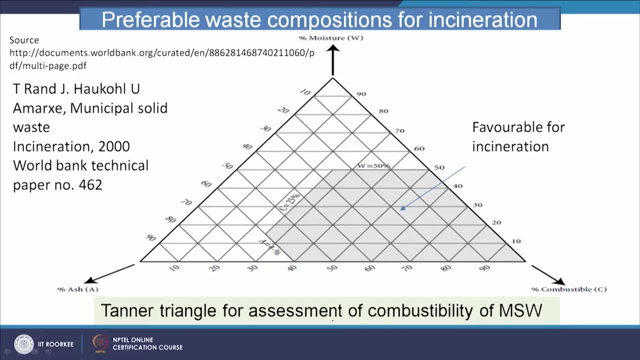 of the materials for incineration. So here diagram shows That this is percentage combustible and another percentage moisture and percentages. this is favourable conditions for incineration, so high carbon content, less moisture and less ash content are more favourable for this. This is the process flow sheet for the incineration. 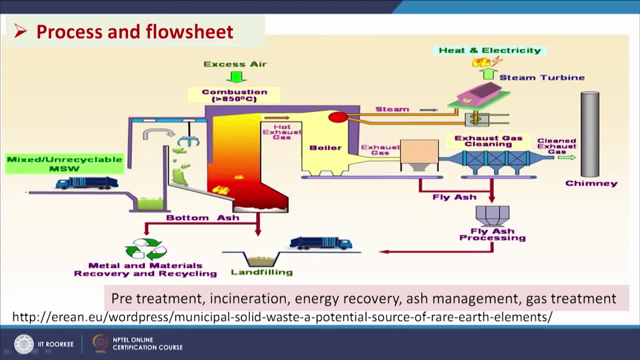 of municipal solid waste, so it is coming here after sorting, so which can be produced and processed, so it is mixed and un-recyclable. MSWT is coming, so here it is going for sorting and then it is coming here, So this material, which is desirable, is entering into this combustion chamber and it will be. 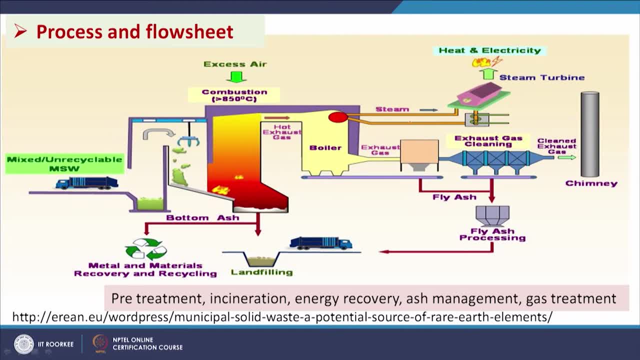 heated, so flue gas will be generated. that will be the heat will be recovered through the steam production and that will be used for the electricity productions or any process steam application, Then this one which is coming from the bottom of this reactor, so that will be containing. 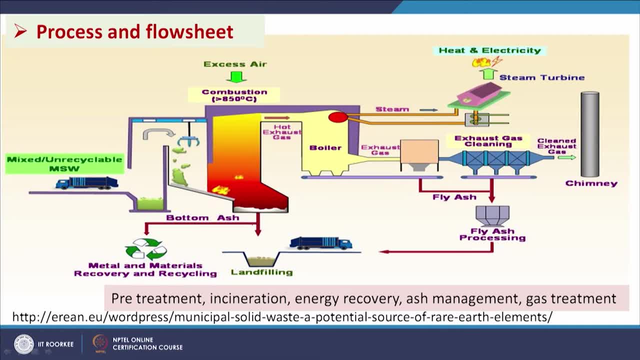 metal and materials and ash content, basically. so it will go for metal and materials recovery and recycling. and where we are getting it is this: hot gas is going to boiler and then we are getting steam and then the bottom part is going for exhaust gas and this is the gas. 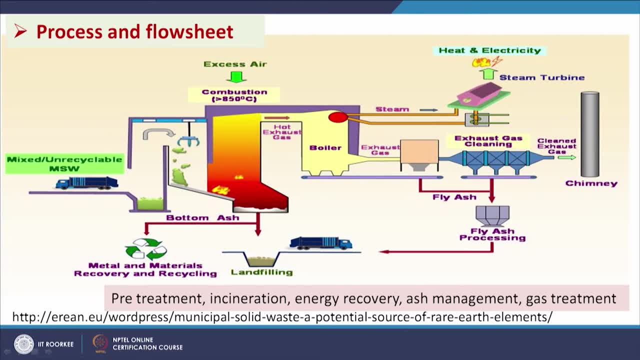 which is coming out After heat recovery. This is the gas which is going through this and then it will be cleaned- so clean there will be some particulates also. those particulates will be separated here in this separator and that fly ash will be processed further for the land filling or through other routes. and 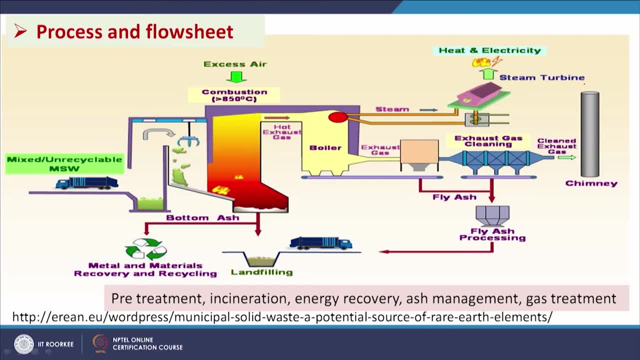 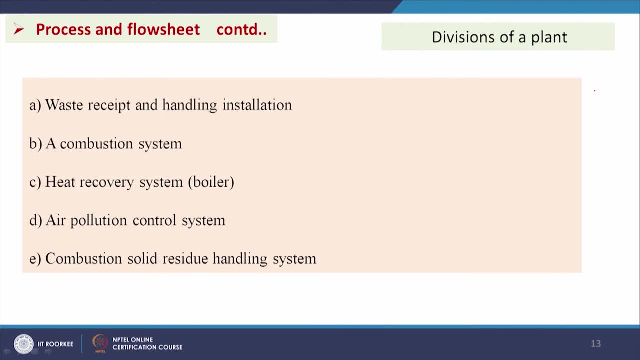 this will be the gas stream that will be cleaned and released to the environment. So this is the process for the incineration method and it has different parts. this incineration plant has different parts like, say, waste receipt and handling installation, then a combustion. 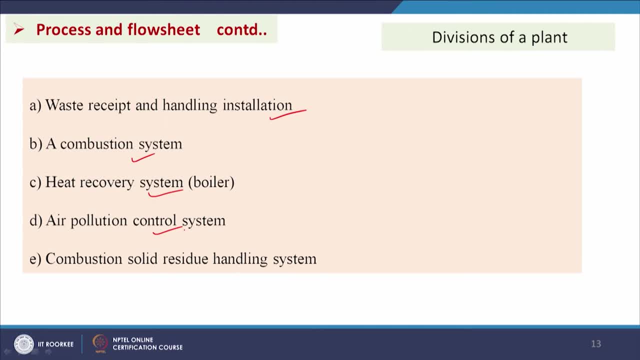 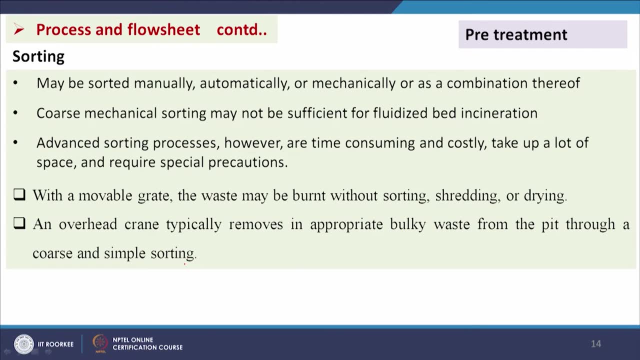 system, a heat recovery system, air pollution control systems and combustion solid residue handling system. So sorting this may be sorted manually. the MSW may be sorted manually, automatically or mechanically, or as a combination thereof. coarse mechanical sorting may not be sufficient. 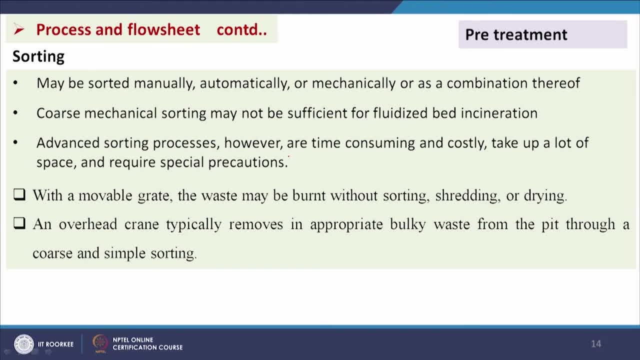 for fluidized bed incineration. Advanced sorting process may not be sufficient for fluidized bed incineration. Advanced sorting process may not be sufficient for fluidized bed incineration. The process is, however, time consuming and costly, take up a lot of space and require. 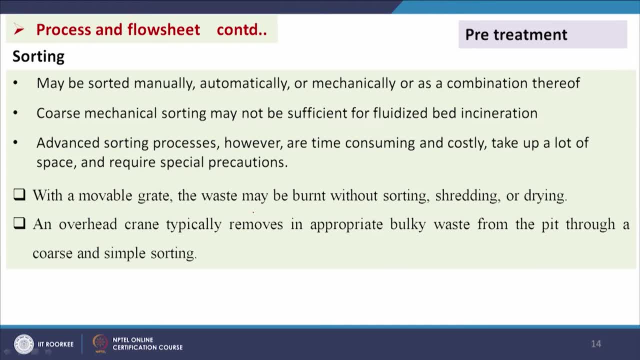 special precautions. With a movable grate, the waste may be burnt without sorting, shredding or drying, So grate firing is implemented in many cases, and overhead crane typically removes inappropriate bulky waste from the pit through a coarse and simple sorting. so that we have shown 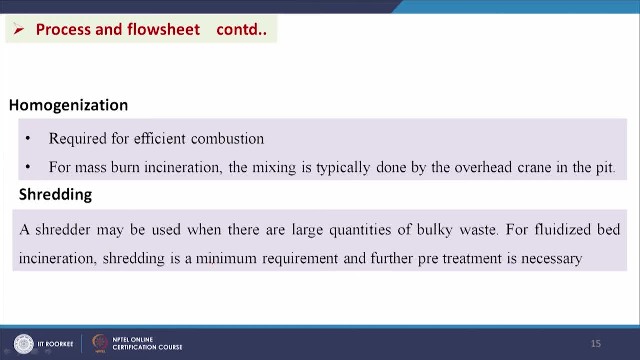 in the in the previous video, previous slide in the previous flow sheet and homogenization. this is required for the efficient combustion for mass burn incineration. the mixing is typically done by overhead crane in the pit and shredding. a shredder may be used when there are large quantities of bulky. 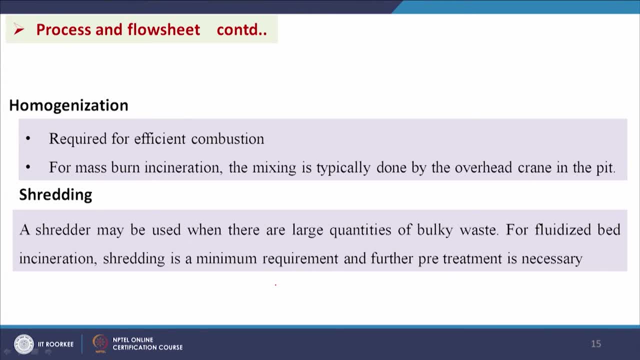 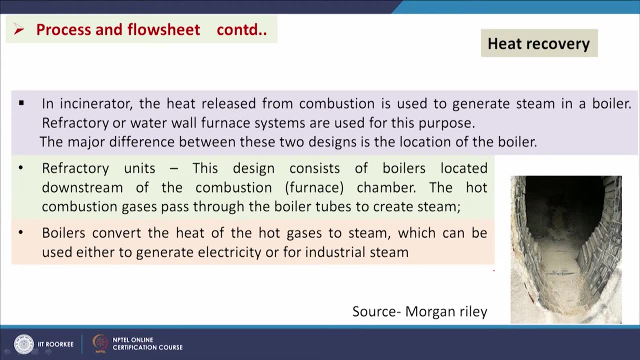 waste for fluorized bed incineration. shredding is a minimum requirement and further pretreatment is necessary. now we are coming to heat recovery. so heat recovery in the incinerator. the heat is released and it is associated with the flue gas and that heat is used for the production of steam. 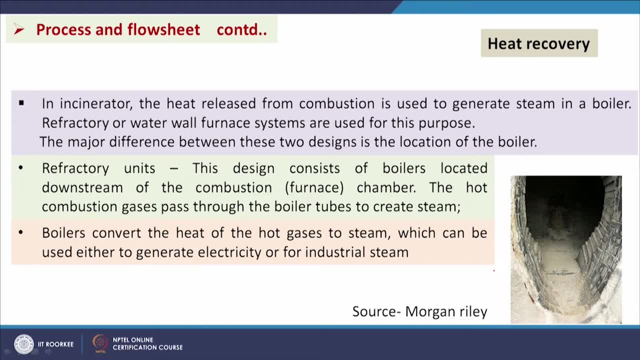 in a boiler. so there are two types of boiler: one is your refractory or and another is your water wall furnace systems. so the major difference between these two. we are coming to heat recovery. so heat recovery in the incinerator. the heat is released and it. 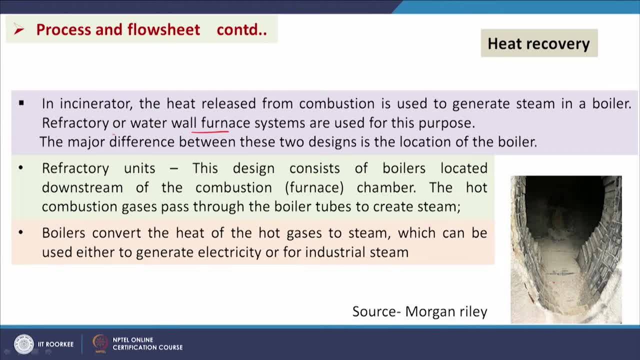 designs is the location of the boiler. In some cases we have one furnace separated by a boiler. So in this refractory furnace where burning or combustion of the material will take place and the flue gas will go out from it and it will enter into a boiler, It. 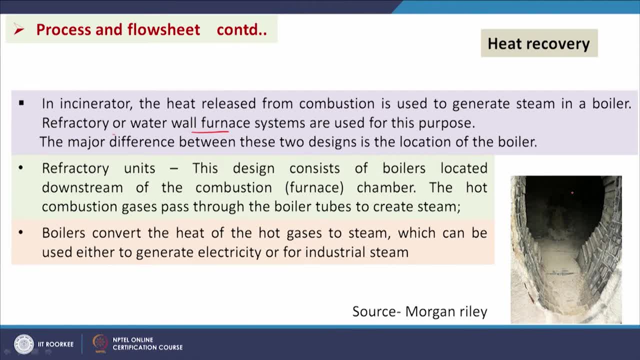 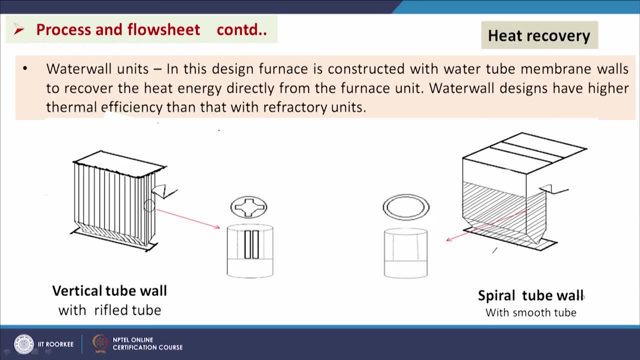 will be in contact with water direct or indirect, and will get steam. So that is one design. Another design is there, that is, water wall furnace. In that case the furnace is constructed with water tube membrane walls to recover the heat energy directly from the furnace. 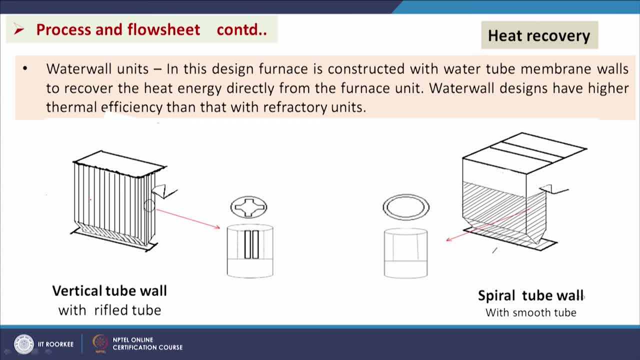 unit. So if it is a furnace unit, so in the wall of the furnace we have water tubes, So directly it is in contact with the flue gas in the furnace itself and then water is converted to steam. So that way, so in book you may get that. 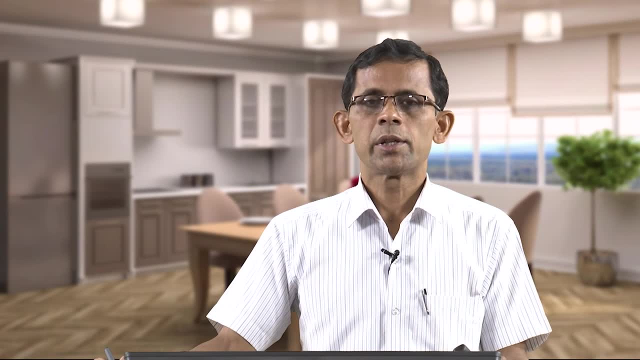 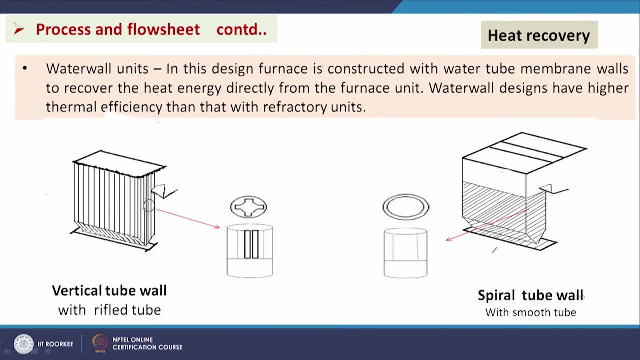 somewhere in the book it is mentioned that only boiler. somewhere it is mentioned that furnace and boiler- So when we use this water wall units, so then it is furnace and boiler- are same. but when we go for refractory unit, then the furnace and boiler are different units. 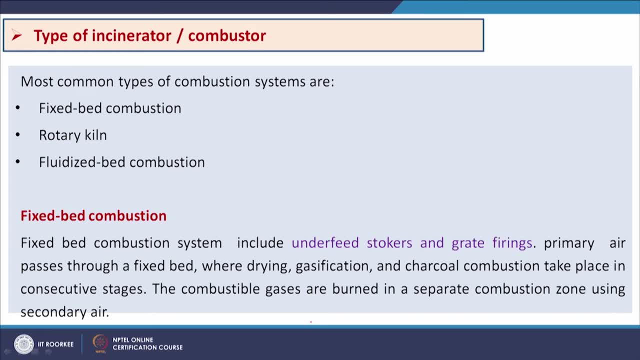 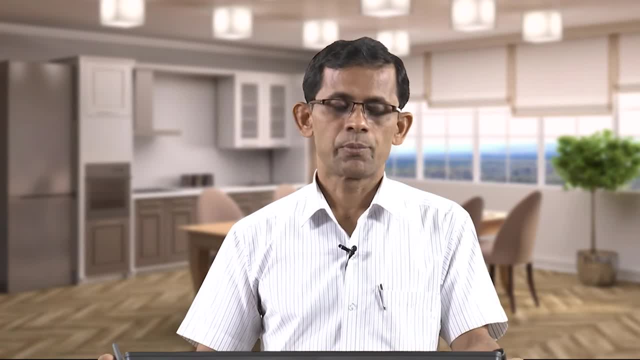 Now different types of combustion system. if we think about the reactor type, then it can be fixed bed combustion, then rotary kiln and fluidized bed combustion, So fixed bed combustion. in this fixed bed combustion system it includes under feed. 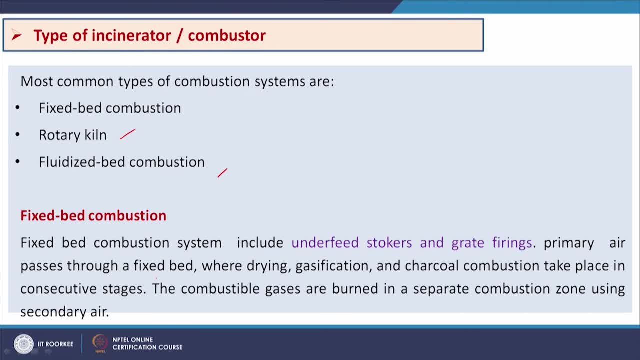 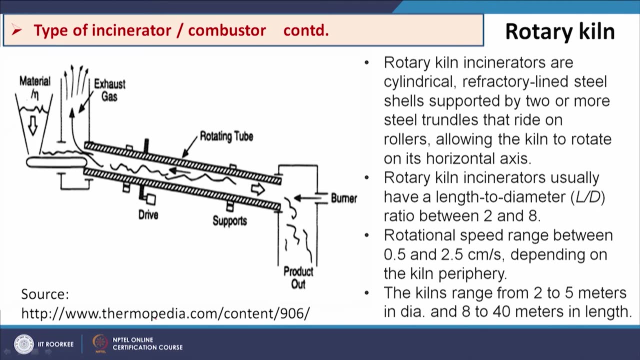 stroker and grate firings, and primary air passes through a fixed bed where drying, gasification and charcoal combustion take place in consecutive stages. The combustible gases are burned in a separate combustion zone using secondary air In rotary kiln as shown here. 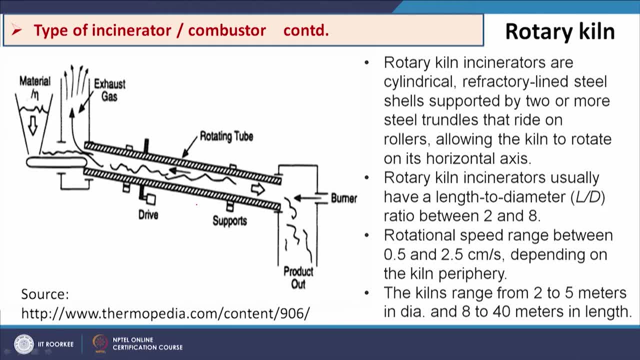 So we have one, We have a rotating tube, so material is coming here and here, the burner initially firing, so then it is going, the flue gas is going, so gradually, temperature is increasing, and so here we are, getting the ash or product out and the gas is going out. 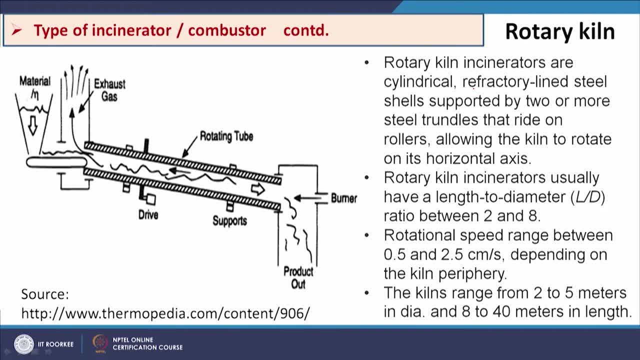 So this hot gas will be used for the heat recovery And rotary kiln. incinerators are cylindrical, refractory lined steel cells supported by two or more steel trundles that ride on rollers, allowing the kiln to rotate on its horizontal axis. 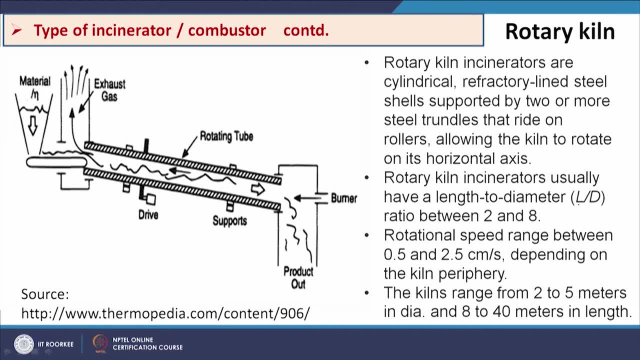 Rotary kiln incinerators usually have a length to diameter ratio between 2 and 8 and rotational speed range between 0.5 and 2.5 centimeter per second, depending on the kiln periphery. The kilns range from 2 to 5 meters in dia and 8 to 40 meters in length. 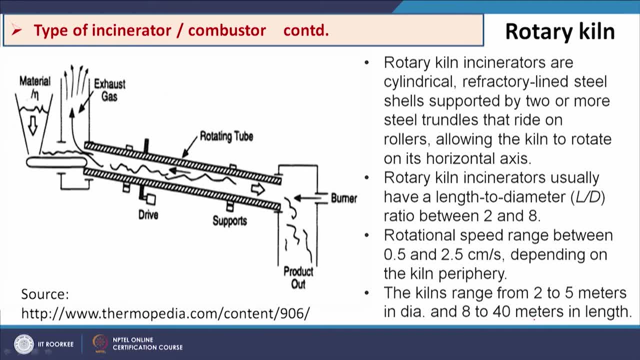 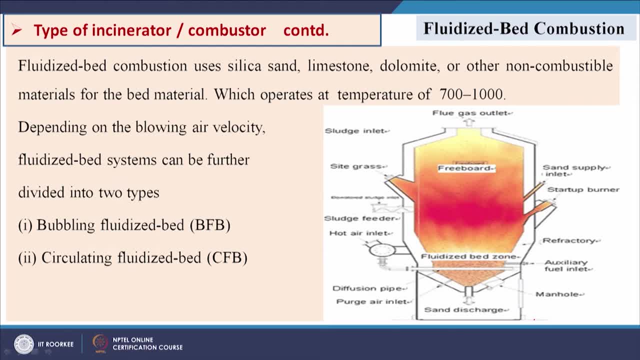 So these are some typical dimensions of the rotary kiln. In case of fluidized bed combustion, we need to use smaller size of the materials. So this is one photographs of this fluidized bed combustor. So here the material is getting entry and here we are sending the air and we have some 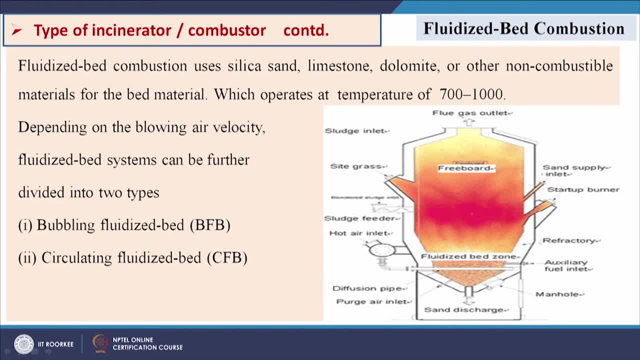 material here. So here we are sending the air and we have some material here. So here the material is getting entry and here we are sending the air and we have some material here. So here the material is getting entry and here we are sending the air and we have some. 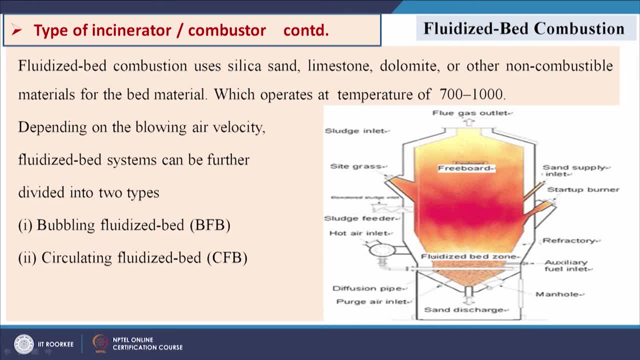 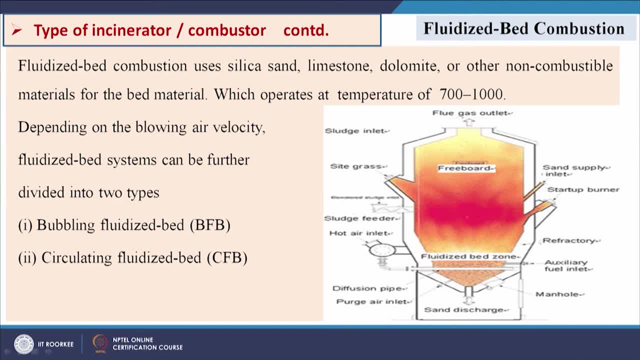 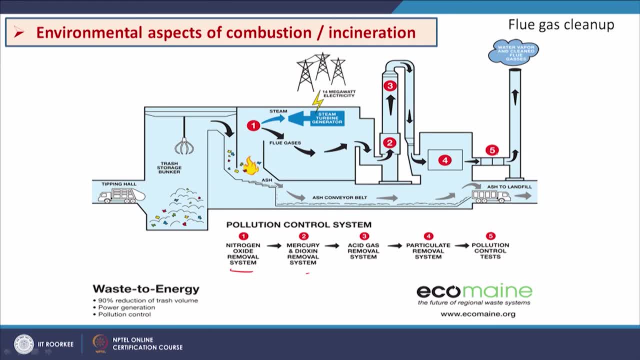 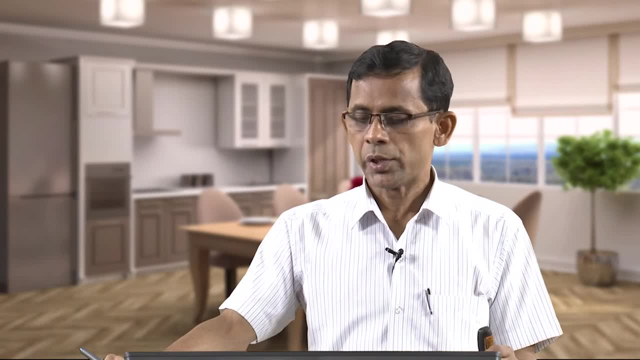 here we are sending the air and here we are sending the air and here we are sending the. We have to measure the pollution control test. that means what is the PM content, what is the NOx, SOx, CO, etcetera concentration is available. that will be continuously monitored. 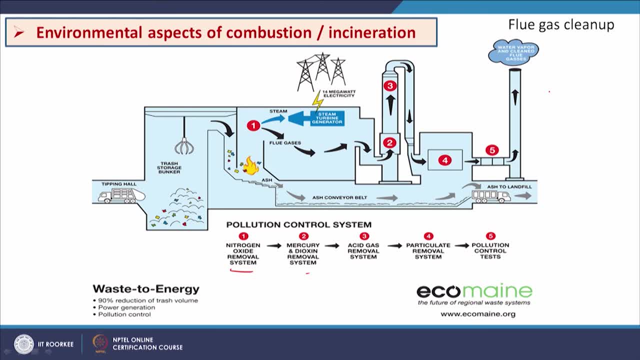 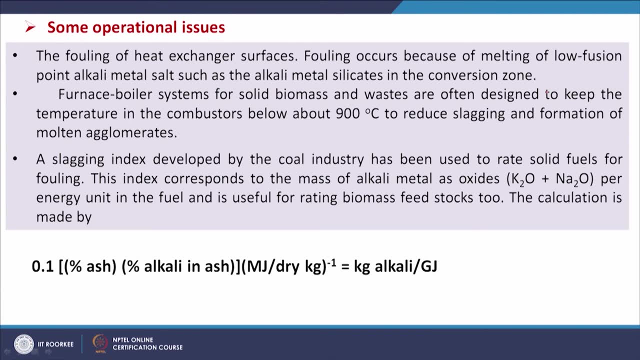 to ensure the environmental quality and to eliminate the emission into the environment. Now some operational issues we will discuss. One important issue is fouling. So why the fouling is taking place? So where heat transfer is taking place in case of furnace or boiler. in that case the 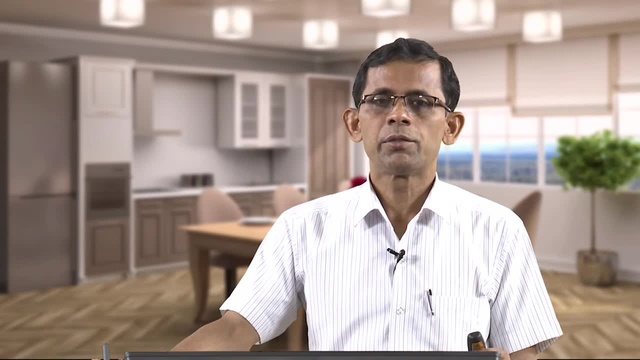 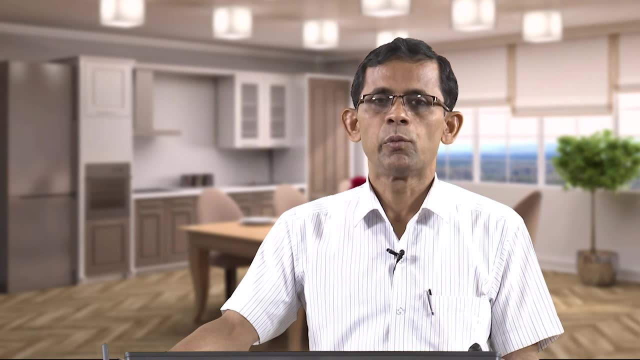 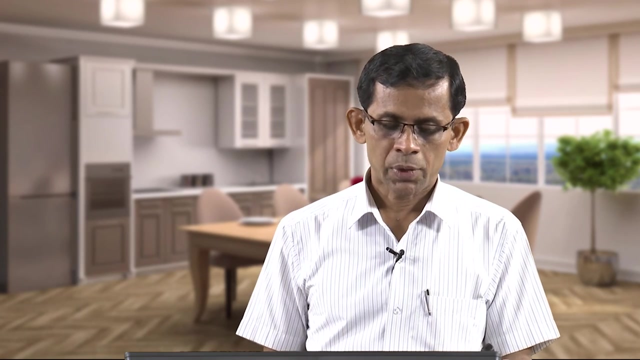 fouling will take place in the furnace or in the boiler if the material, the waste material, is having very high ash content and ash is being molted. it is in the molten stage it is forming a slag, so that will create a layer on it and the fouling will occur. 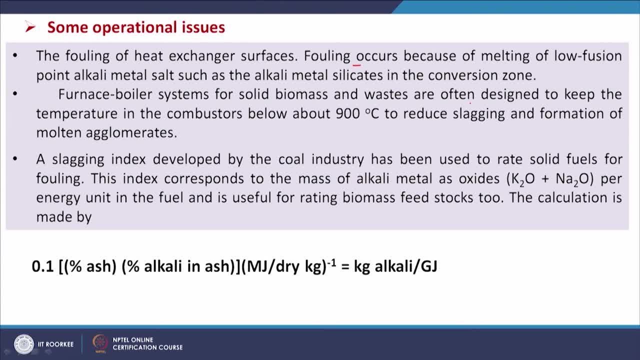 So furnace boiler systems for solid biomarkers, Amass and waste, are often designed to keep the temperature in the combustor below about 900 degree centigrade to reduce slagging and formations of molten agglomerates. So that is one way of technique to avoid this type of formation. 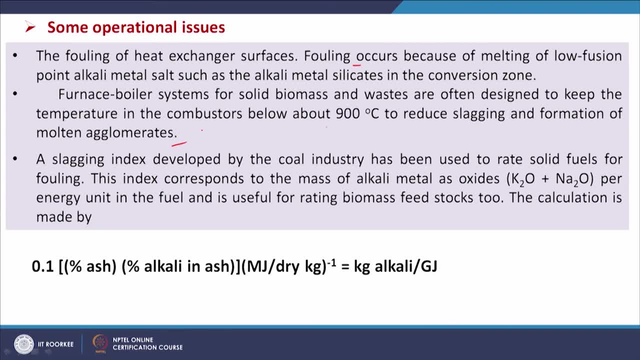 But why this agglomeration takes place. certain theoretical consideration is there and that we are discussing now. So the slagging index develop by the coal industry has been used to rate the flue. When this slagging index is developed by the coal industry has been used to rate the flue. 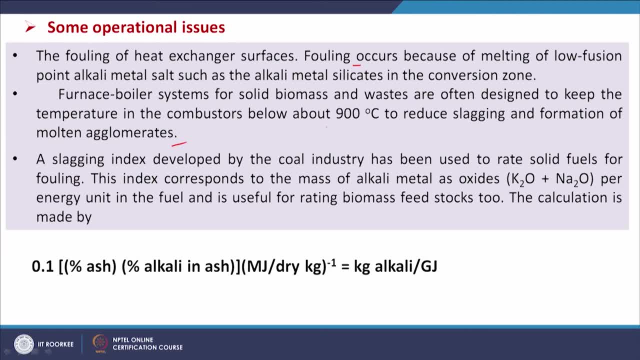 This is a very interesting example. So in urban area, for example in the south of India, there are some best known smelters, solid fuels for fouling. This index corresponds to the mass of alkali metal as oxides, that is K2O plus Na2O per energy unit in the fuel and is useful for 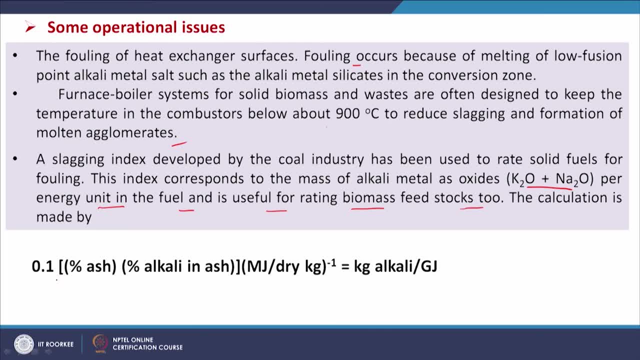 rating biomass feedstocks too. The calculation is made like this: 0.1 into percentage ash, into percentage alkali in ash, that is, in mega joule per dry kg is equal to kg alkali per giga joule. So this is the way, on the basis of percentage of alkali in ash and total percentage. 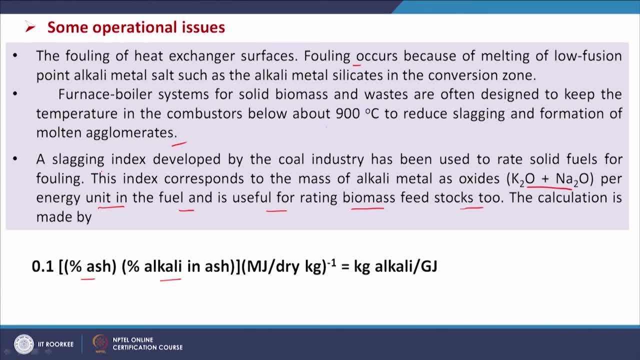 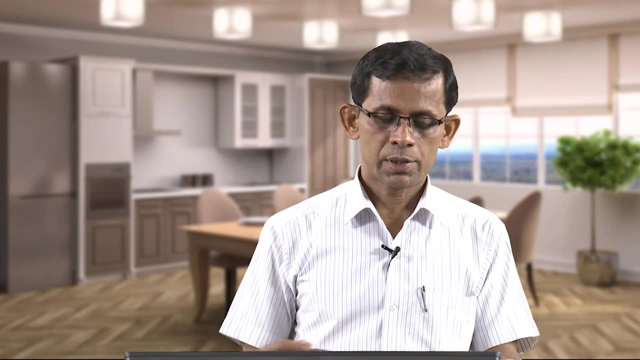 of ash, we can calculate the slag index, and this alkali means K2O and Na2O. So knowing the percentage of the K2O and Na2O, or we can say that knowing the composition of the ash, we can get some idea about the slagging index. and this and slagging index. 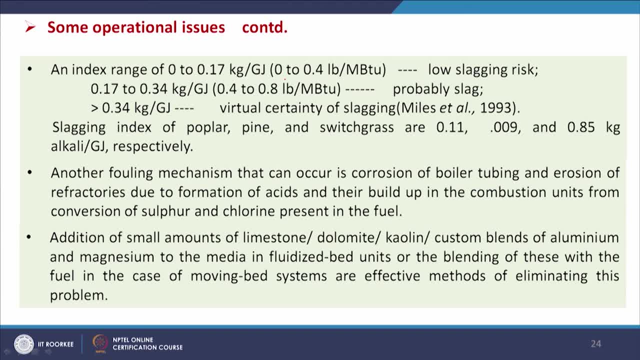 range of 0 to 0.17 kg per giga joule, or 0 to 0.4 lb per mbtu. that is low slagging risk, and 0.17 to 0.34 unit, that is probably slag, and greater than 0.34 unit, that is kg per giga joule. that 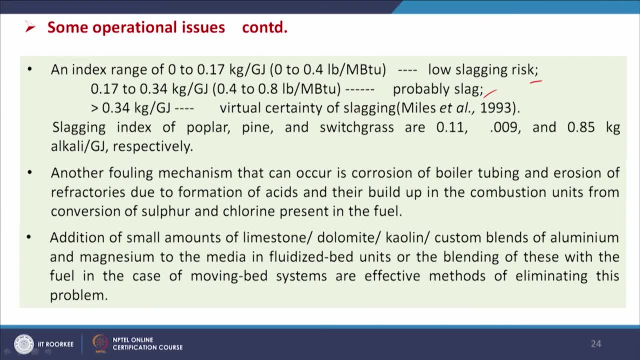 is virtual certainty of slagging, So that will be. there is a good possibility of slagging, So there is slagging index of poplar pine and switchgrass are given here. So another fouling possibilities. This is because of the presence of, you know, the acid gases, So that the corrosion of 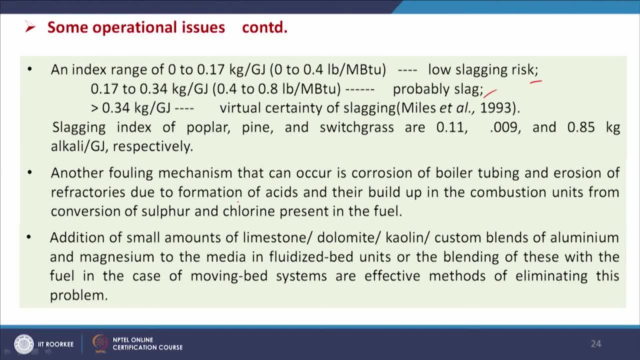 the boiler tubing and erosion of the of the refractories due to formation of acids and they are build up in the combustion units from conversion of sulphur and chlorine present in the fuel. And for avoiding this, some metal oxides are added, like, say, limestone, dolomite, kaolin and castor, blends of aluminium and magnesium. 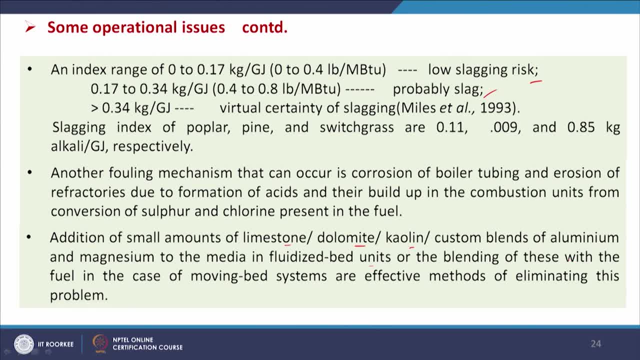 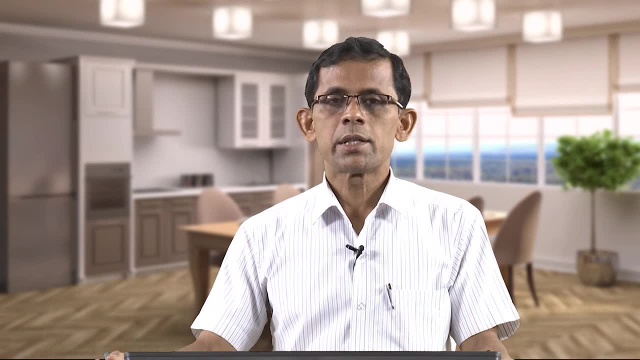 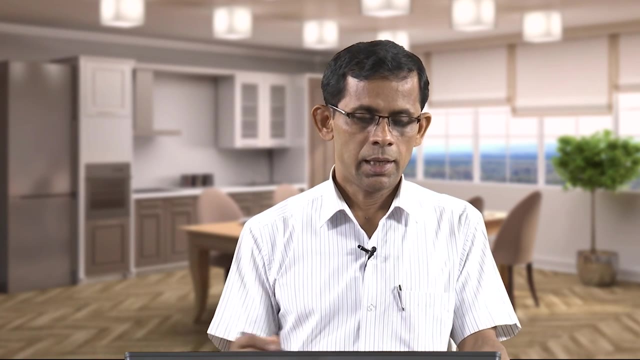 to the media and fluidized with units, or the blending of these with the fuel in the case of moving with systems, are effective methods for eliminating this problem. So chloride and sulphur is captured by these materials. some some waste incineration plants plant are built in India or provided in this slide, like say, Narela, Delhi, Ramki, Gazipur. 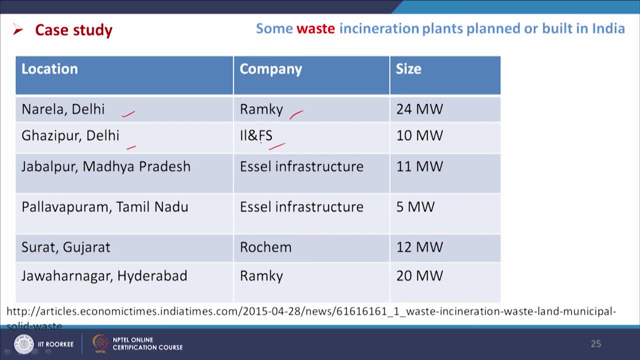 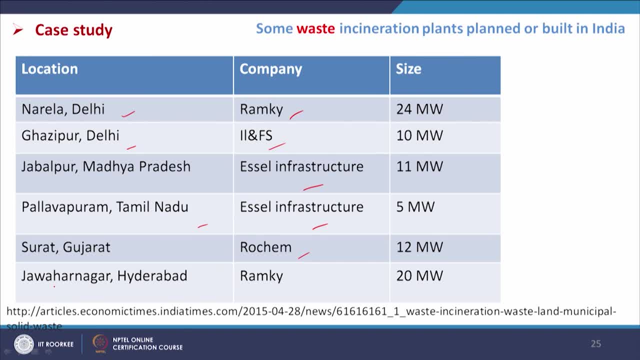 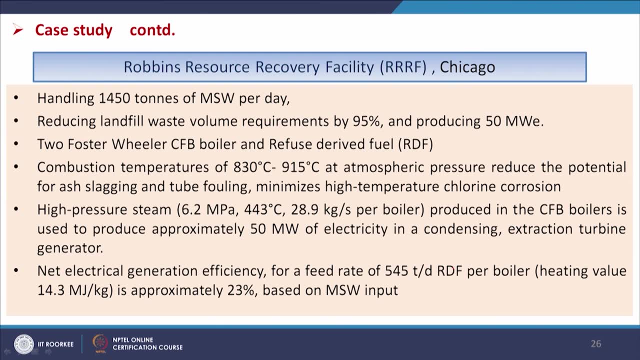 Surat, Gujarat, Rochim, and Johar Nagar, Hyderabad, Ramki. so these are some size, these are some capacity of the incineration waste plants. Another case study is Robbins Resource Recovery Facility at Chicago. so here handling is 1450. 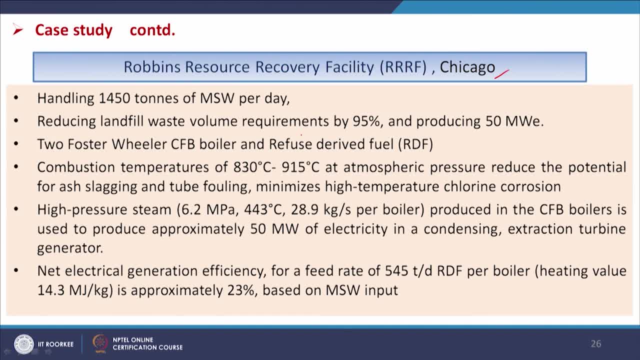 tons of MSW per day, reducing landfill waste volume requirements by 95 percent and producing 50 megawatt electricity, two foster wheeler CFB boiler and refuse-drived fuel. it has two foster wheeler CFB boiler and using refuse-drived fuel, that is, RDF, and combustion temperatures. 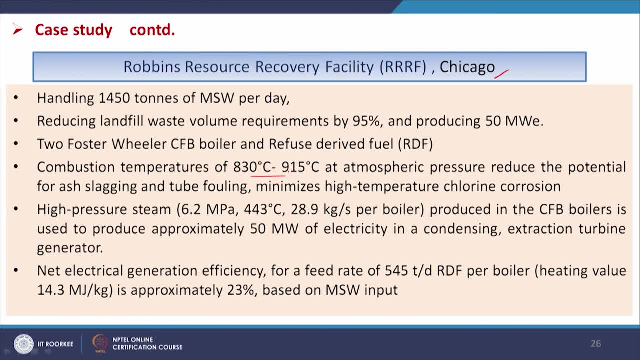 of 830 to 915 degree centigrade at atmospheric pressure. Reduce the potential for ash slagging and tube fouling. minimizes high temperature, chlorine corrosion, high pressure steam at a 6.2 megapascal for 43 degree centigrade, that is, 28.9 kg per. 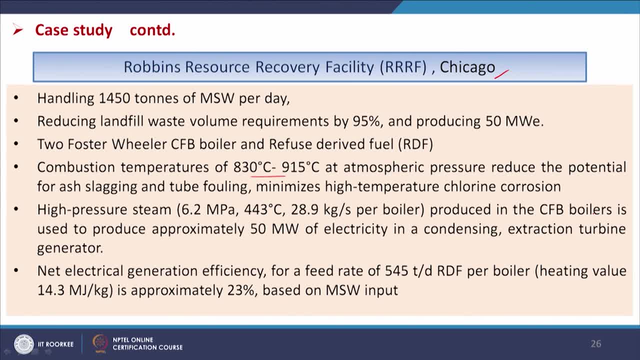 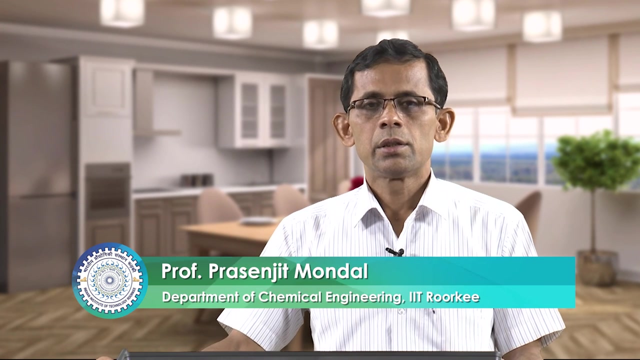 second, per boiler. that produced in the CFB boilers is used to produce approximately 50 megawatt of electricity in a condensing extraction turbine generator. net electrical generation efficiency for feed rate of 545 ton per day RDF per boiler. So these are some case study. so we have made some discussions on the incineration.